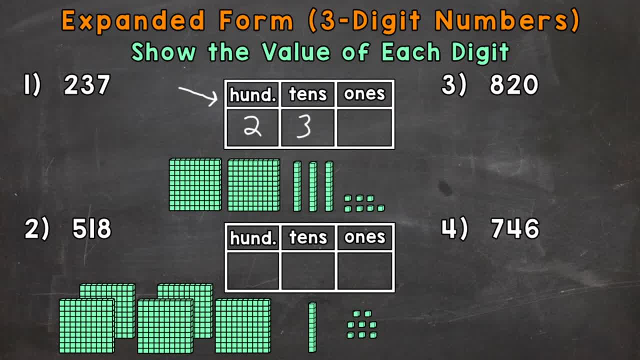 place, a 3 in the tens place and a 7 in the ones place. So again for expanded form, we want to show the value of each of these digits and we'll start with our greatest valued digit, So the digit furthest to the left. 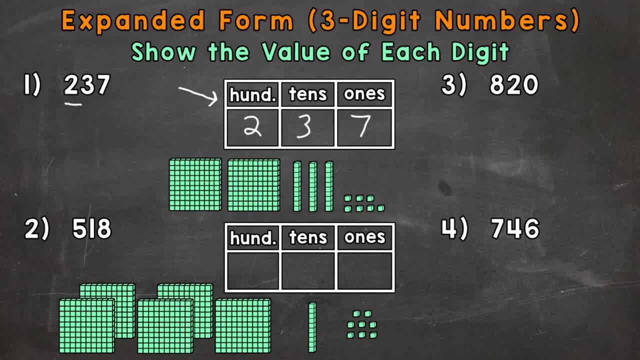 This 2.. So that 2 is in the hundreds place, So it has a value of 200.. It's representing two groups of 100 and we can see with our place value blocks, right here we have 100, 200 to give a visual of the. 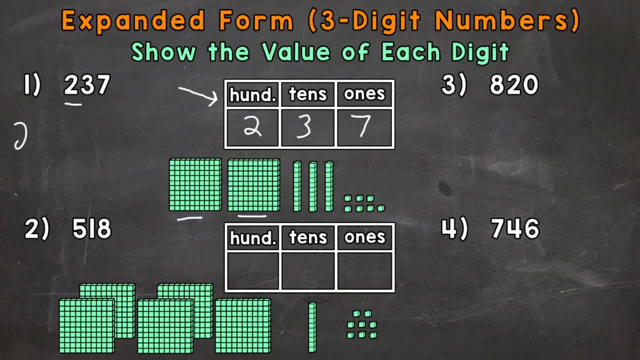 value of that digit. So we'll start by writing 200.. Again, the value of the 2 is 200, because that 2 is in the hundreds place, Plus let's do the value of the 3.. So that 3 is in the tens place. It represents 3 groups of 10 where we 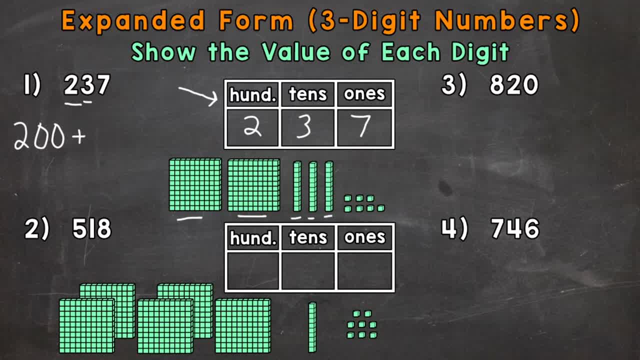 have 1,, 2, 3 groups of 10 right there represented by those place value blocks, and the value of that 3 is going to be 30.. So 200 plus 30 plus next we have the 7.. So the value of the 7 is 7.. That's. 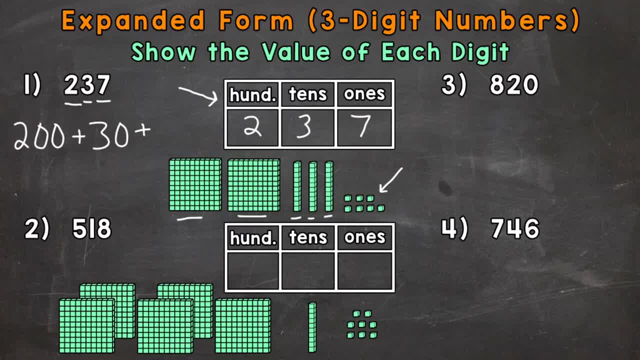 7.. It represents 7 ones, So we'll put a 7 here. So to recap, the 2 has a value of 200 because it's in the hundreds place, The 3 has a value of 30 because it's in the tens place, and the 7 has a value of 7. 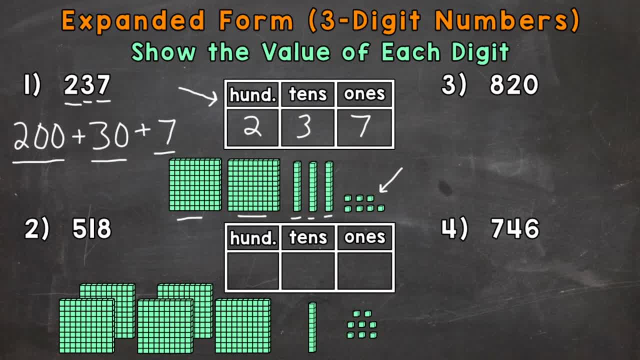 because it's in the ones place. So let's go on to number 2, where we have 518.. So we have a 5 in the hundreds place, A 1 in the tens place, 1 in the tens place, One in the tens place. 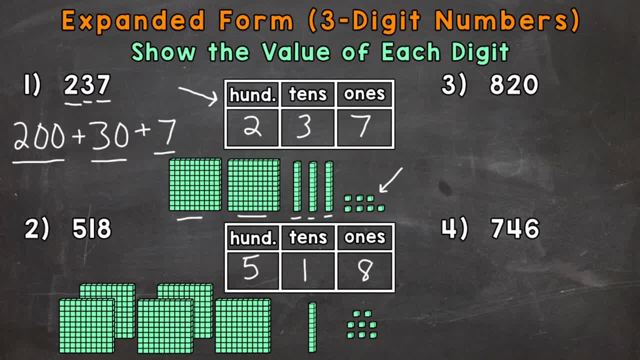 and an 8 in the ones, so that 5 has a value of 500. it represents 5 groups of 100, which again is 500. so we have 500 plus the value of the one. that one represents one group of 10, which has a value of 10, plus the 8 which represents